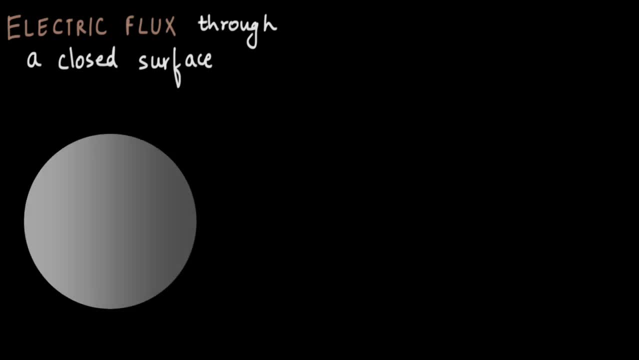 a closed surface where if we had a closed surface like this, a closed spherical surface and let's say we had a positive charge in the center, we know that the flux that is going through the surface would be given by the closed surface. integral of the dot product between the 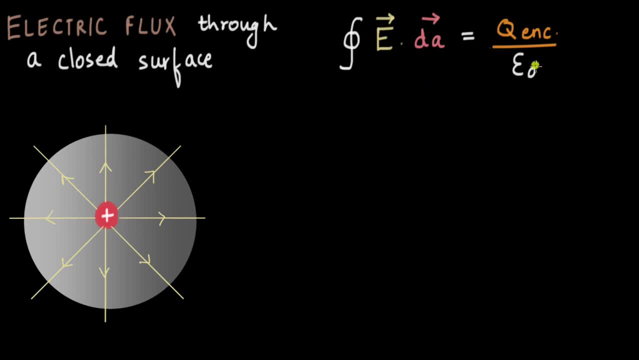 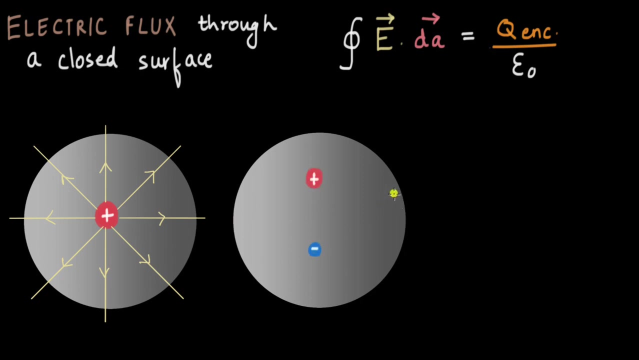 electric field and area which equals the amount of charge enclosed in that surface divided by epsilon naught. Now what if, just instead of a single positive charge, a monopole of electric charge, you take an electric dipole inside the Gaussian surface, just like this? Now what do you think the electric flux would be? Pause the video. 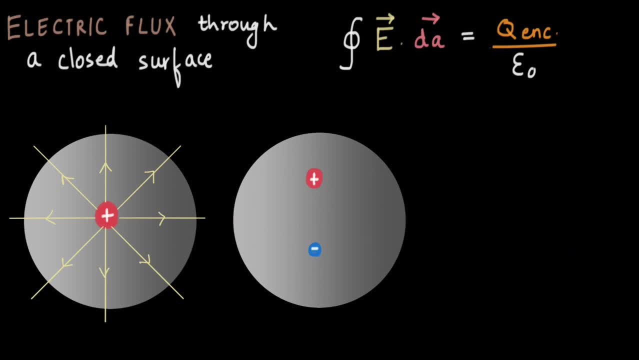 and think about it. All right, I'm sure you'll agree that the electric flux in this case would just be zero, because your enclosed charge would come out to be zero. you have a plus Q and you have a minus Q, So let's look at the field lines. This is how the field lines would look like You. 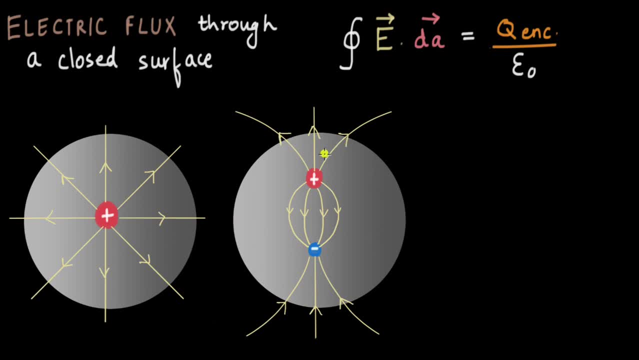 can see that the number of field lines that are leaving the surface is equal to the number of field lines that are entering the surface from the other side. So no matter where you place your electric dipole inside the sphere, your flux will always come out to be a zero. Now let's bring back. 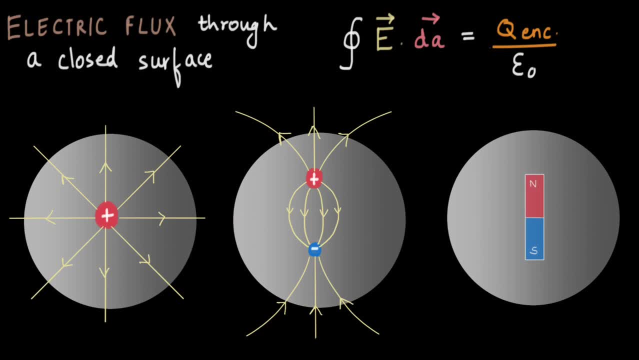 our magnetic dipole into the picture And this is how it can look like. Again, pause the video and think about what would be the magnetic flux in this case. All right, so the magnetic flux in this case would be zero, Because there are no monopoles over here. 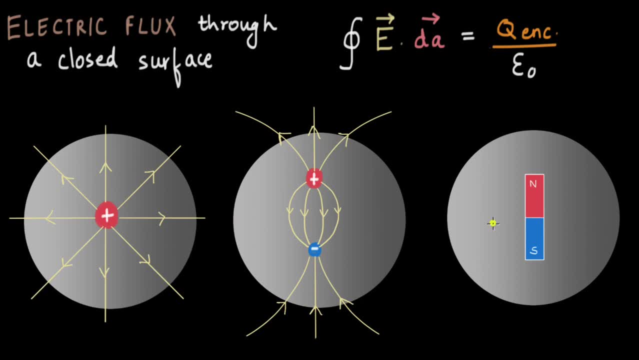 we are taking a magnetic dipole And just like how flux for an electric dipole was zero, similarly the flux for a magnetic dipole is zero. We can even have a look at the field lines and see how geometrically similar they are. We can see that the number of field lines that are 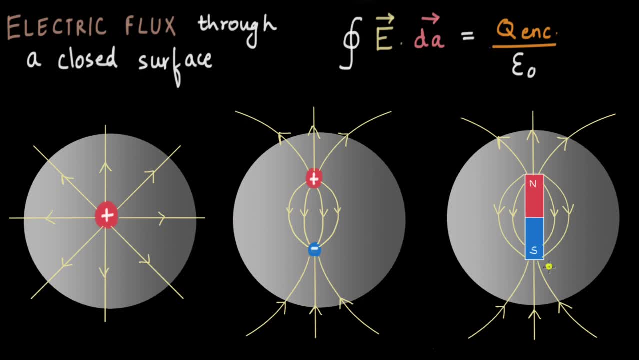 leaving the surface is equal to the number of field lines that are entering the surface. So now we can think about Gauss's law of magnetism, just like Gauss's law of electricity, only if we had dipoles. And just like it doesn't matter where you place the electric dipole inside the surface. 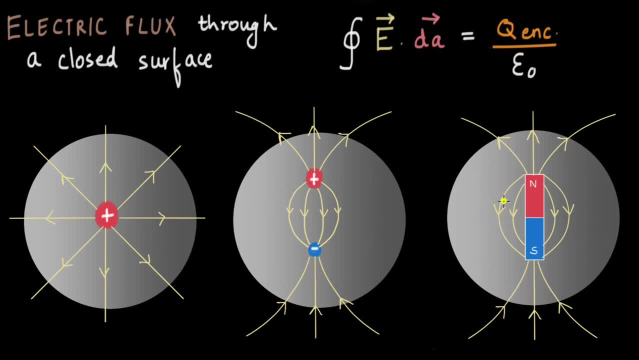 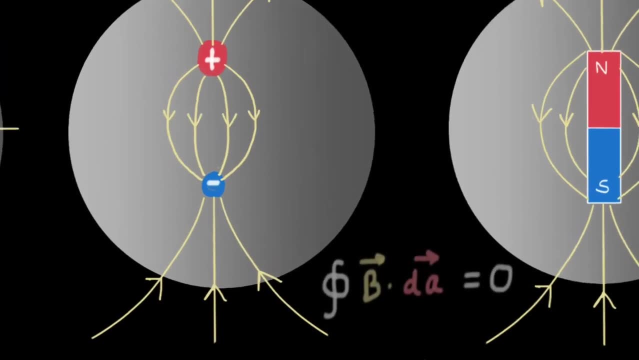 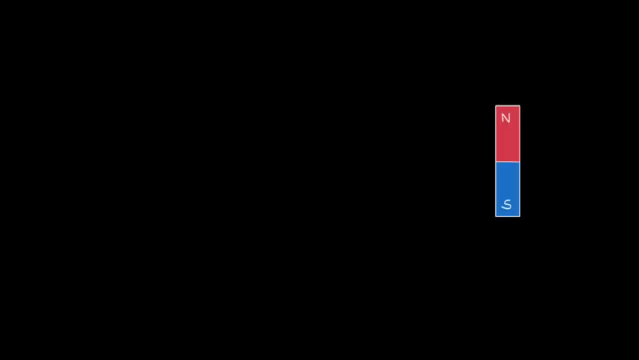 your flux would be zero. Similarly, it wouldn't really matter how you place the bar magnet inside the surface, you will always get the magnetic flux to be as zero. Now what if we kept the bar magnet outside the surface somewhat like this. let's say this is: 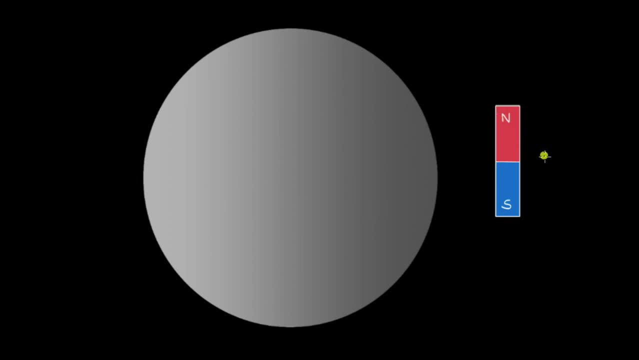 your surface and your bar magnet is just right next to it, outside of it. So the magnetic field lines in this case would look like this: Now, over here, we can still see that the number of magnetic field lines that are entering the surface, and that would be two in this case- this is the first. 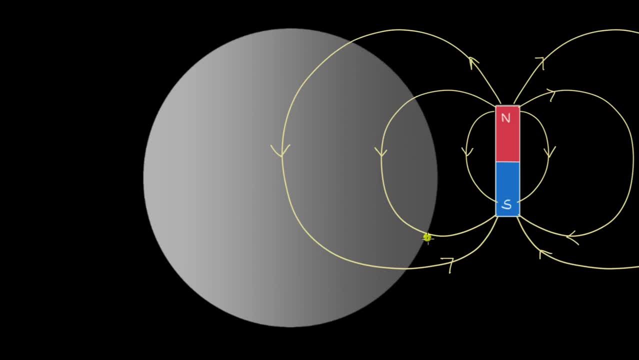 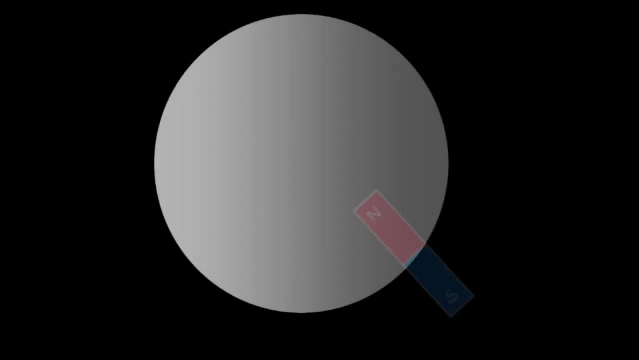 one. this is the second one. they equal the number of field lines that are exiting the surface. So the net flux is still zero. in this case Let's check if the magnetic flux is zero. for a different case, Let's say we move around the magnet and we keep it in this way Half of the 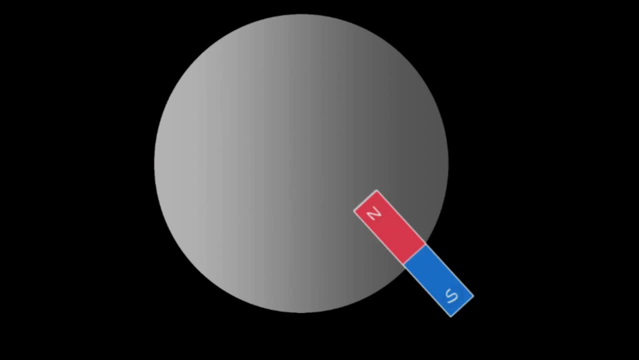 magnet is inside and half of it is outside, And the field lines in this case would look like this: Now, what do you think the magnetic flux would be? Again, pause the video and think about it. Now it turns out that even for this case, 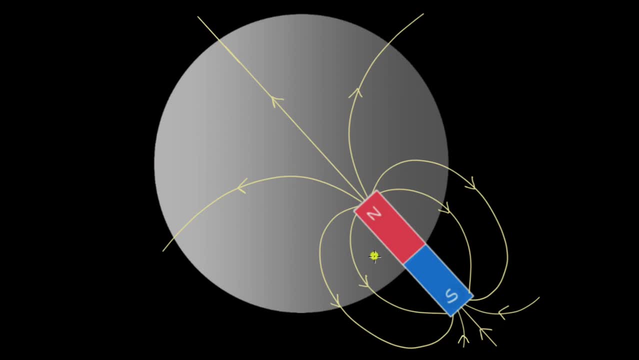 the magnetic flux is zero. You could think that because half of the magnet is inside and half of it is outside, this would be similar to saying that the positive charge, a positive charge, would be inside and a negative charge would be outside. But the key point over here is that magnetic field. 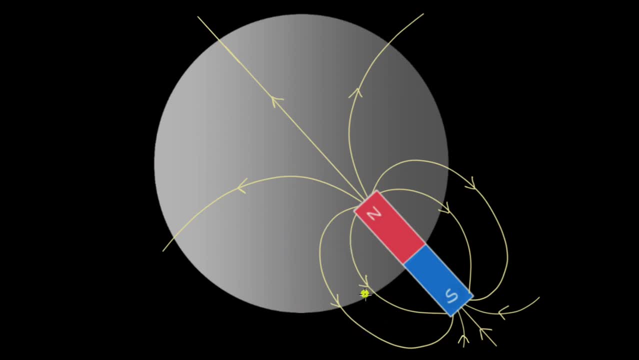 lines form closed, continuous loops, So the field lines, even inside the magnet, go from south to north pole, And this is how they look like Now. if we look closely, we can see that the number of field lines that are leaving the surface 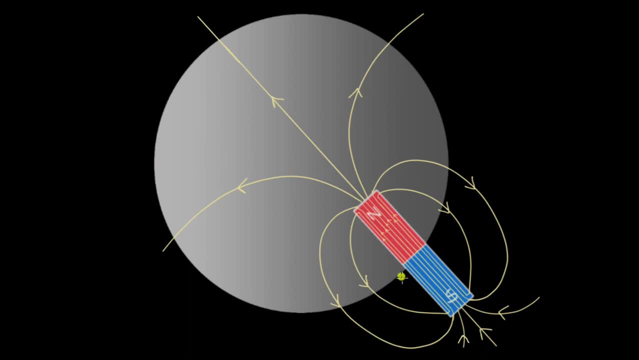 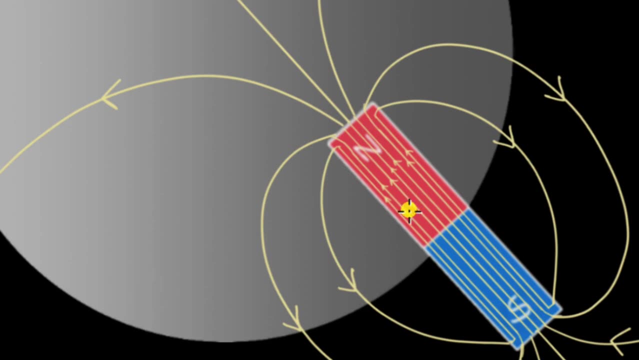 and that would be five in this case. they equal the number of field lines that are entering the surface from inside the magnet. And we can go on to say that this part right here, the part that is near the surface, we can say that this can be a south pole, because, after all, 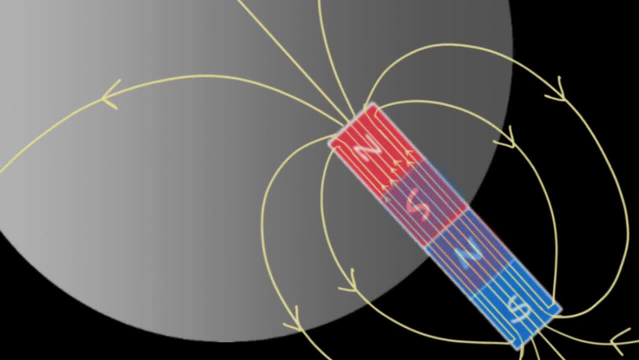 the field lines are going towards the north pole From this region. Now we can say that, because we have a north pole and a south pole inside the magnet, this is very similar to having an electric dipole in the same orientation, So an electric. 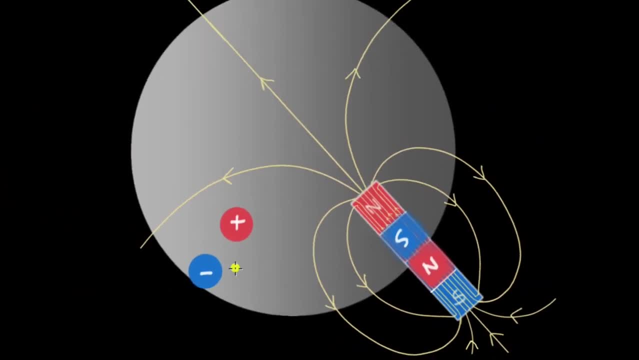 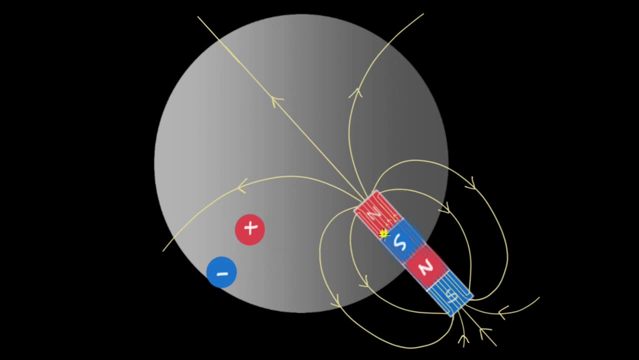 dipole would just look like this, And we know that whenever there is an electric dipole inside the surface, the flux for that would be zero. Similarly, if you have a magnetic dipole inside the surface, the flux for that will be zero. All right, So in this video we looked at: 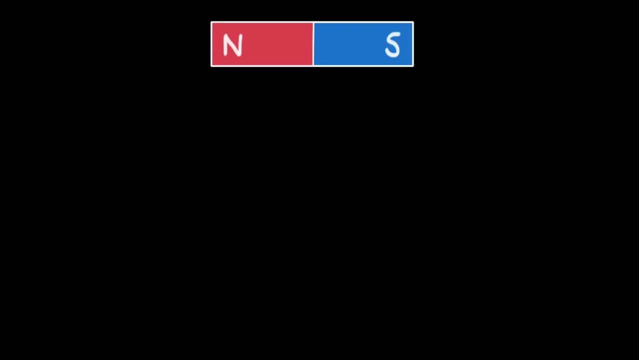 how to take a piece of bar magnet and you break it into smaller pieces. instead of a separate north pole and a south pole, All you get are newer pieces of small magnets, And just like how the flux for an electric dipole came out to be zero, no matter where you place it inside the Gaussian. 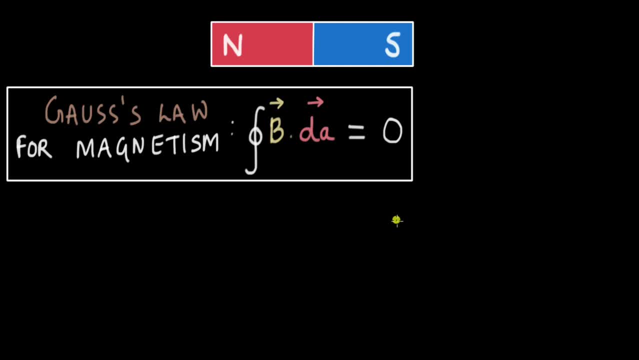 surface. Similarly, the flux for a magnetic dipole also came out to be zero. And we kept the dipole inside, outside, and we kept it half inside and half outside. In all the cases it came out to be zero. Now, if we compare Gauss's law for 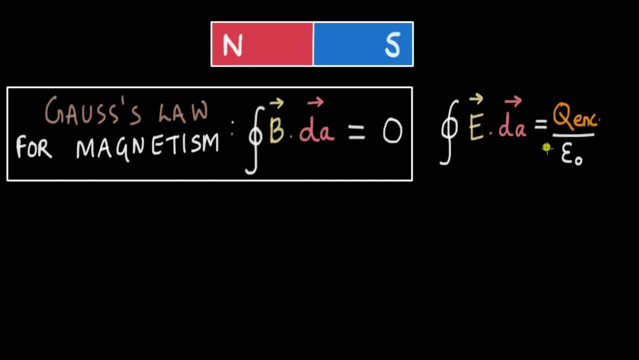 magnetism. with Gauss's law for electricity we can see a noticeable difference. We can see that there is something on the right-hand side for Gauss's law of electricity And that is because there is a monopole of electric charge. You can see a single positive charge and a single negative. 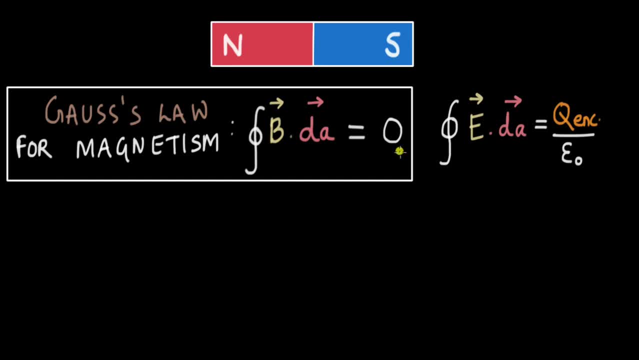 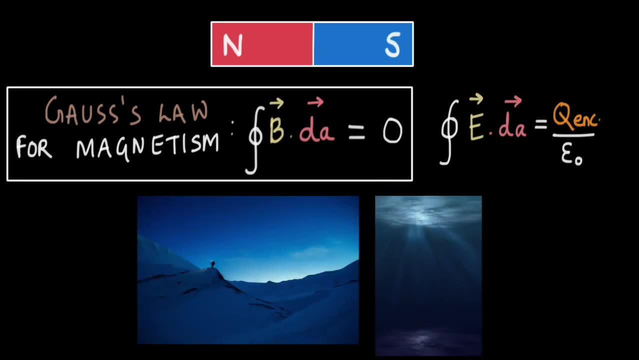 charge, But we can never see a single north pole and a single south pole. So therefore you see a zero over here. Now it turns out that scientists have been searching for a magnetic monopole for almost 90 years now, And they have been to the north pole, they have been to deep underwaters. 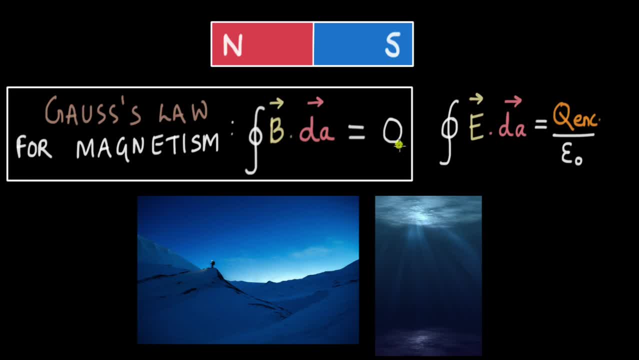 but they haven't been able to find one. And imagine if they do find one. firstly, the right-hand side of this equation will change This equation. the Gauss's law for magnetism will look very similar to Gauss's law for electricity. You will have something like a magnetic charge. 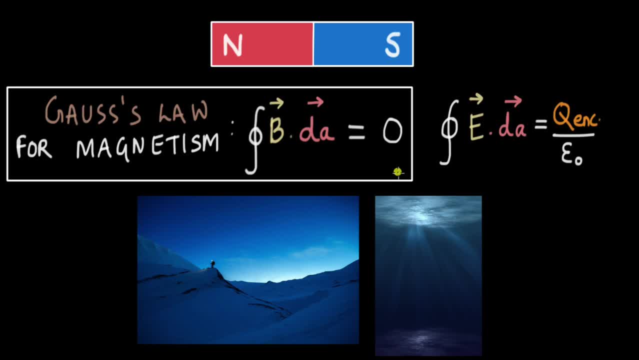 over here And the entire set of Maxwell equations will become beautifully symmetric. We will talk about Maxwell equations in depth in our coming videos.